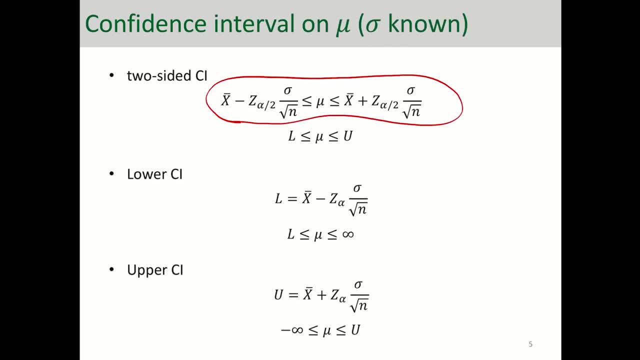 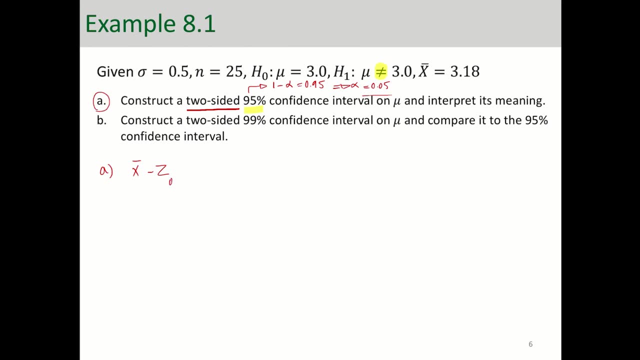 confidence interval minus Z of alpha over 2, Z of alpha over 2. since alpha is 0.05, it's going to be Z of 0.025 times Sigma over square root of n, and upper limit is X bar plus Z of 0.025 times Sigma over square root of n. now, if you replace these: 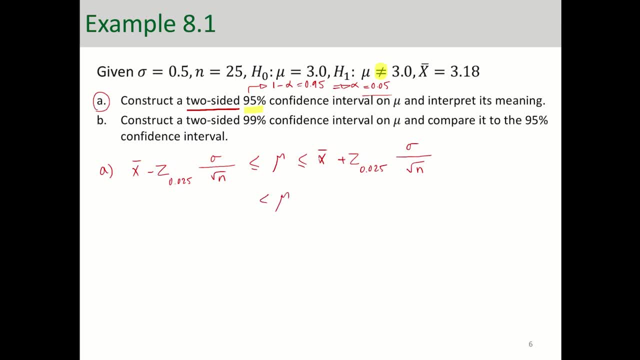 parameters with the numbers. mu is between: X bar is 3.18 minus. this is Z value, as we talked about before- you can read it from the table- is 1.96 times 0.05. Sigma is point 5 and square root of n is the square root of 25 and we're going to. 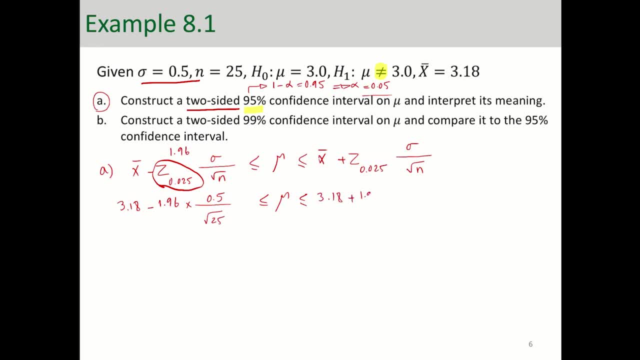 have the right-hand side or the upper limit, and when you calculate and do the math here, you will see that confidence interval, and 95 percent confidence interval, is between 2.984 and 3.376.. So how do we interpret this? What does that mean? Well, this example. 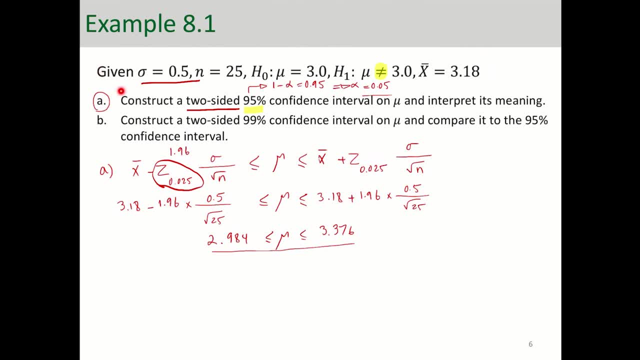 is, if you remember, is the continuation of the GPA example. Essentially, we're hypothesizing whether the average GPA of the university is 3.0 or is not equal to 3.0. Based on the sample that we collected- sample of 25- and this average that we took the confidence. 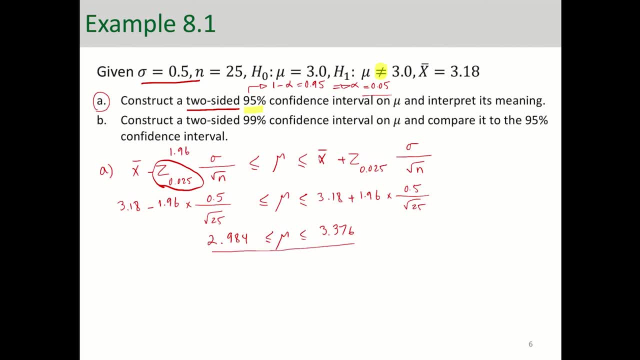 interval is between 2.98 and 3.37.. That means with 95% probability the average GPA of the university is between these two values. That's the meaning of confidence interval. So let's write that down: With 95% probability the true mean of GPA is between 2.984 and 3.376. 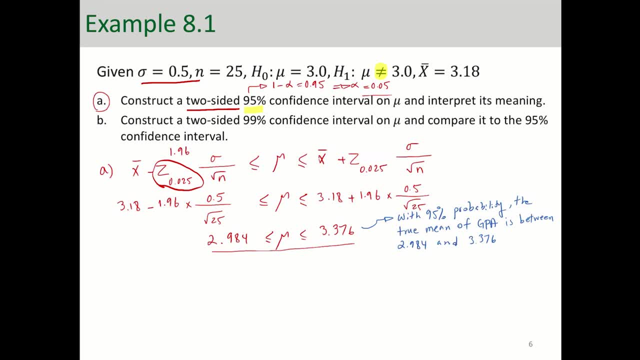 So that's the meaning of confidence interval. So let's write that down. So let's write that down. So that's what this means. So essentially providing that interval or bracket on the population mean. For part B it says: construct a two-sided 99% confidence interval in mu and compare it with 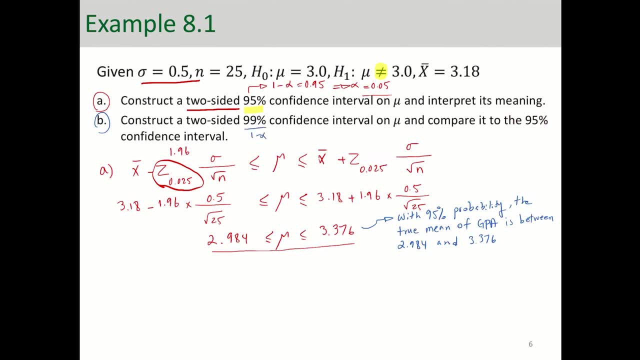 the 95%. So now 1 minus alpha is 99%, meaning that alpha is 0.01.. So what is going to change from part A to part B? So what is going to change from part A to part B? So what is going to change? 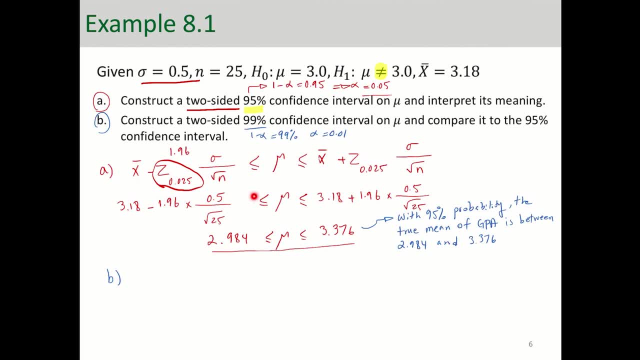 from part A to part B Still is a two-sided. The only thing that is going to change this Z value is going to be Z of 0.005.. Z of alpha over 2 is going to be Z of 0.005, and that is equal to 2.57.. Now 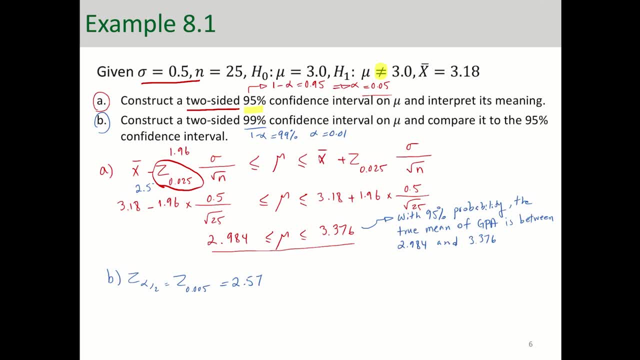 if I change these values to 2.57, and this one also 2.57, and redo the calculations, I'm going to end up with mu between 2.92 and 3.43.. Now how do we interpret that? Very similar to the way we interpret the. 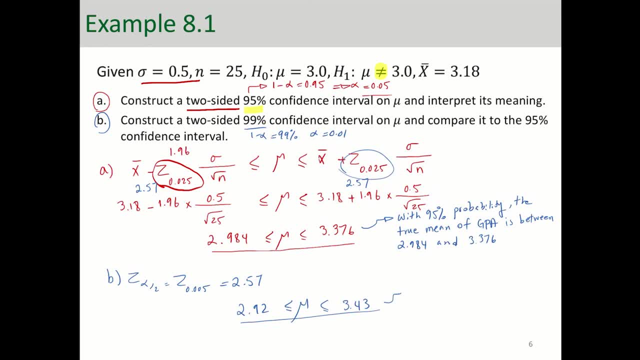 result in part A. Now what we say is: with 99% probability, same statement. with 99% probability, the average GPA is between 2.92 and 3.43.. So what do you realize here by comparing these two confidence intervals? 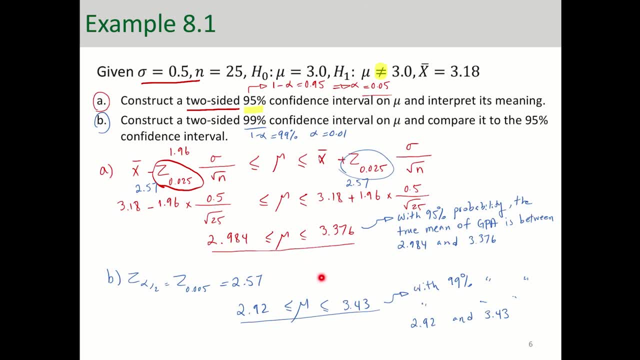 This confidence interval is wider, Both. this value is more than this value and this value is less than this value. So it's a wider confidence interval. it's a wider interval And it makes sense, because now you're saying, with 99% probability, the average GPA is. 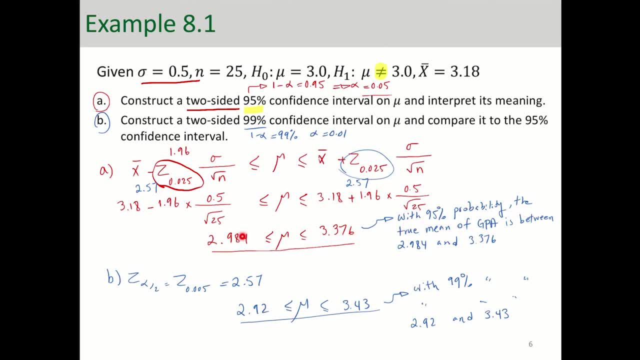 between these two. Here you were saying: with 95%, probability is between: So if you're increasing the probability, you are going to have a wider confidence interval. And this is kind of interesting because you're saying, well, I'm going to have a higher confidence interval. So 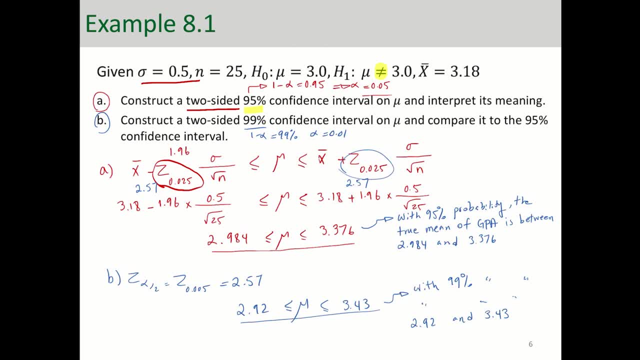 And the face of it is counterintuitive, but when you think about it, it makes sense. As you increase the confidence level, the confidence interval is going to get wider, And we'll talk about that more. So let's look at another version of this example. 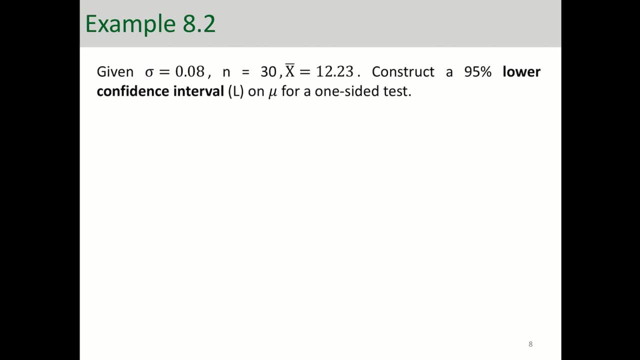 Here we have a sigma which is the standard deviation of the population, and it's 30, x-bar is 12.23.. And we want to construct a 95% lower confidence interval. So in this case it looks like we probably had an alternative hypothesis of one-sided 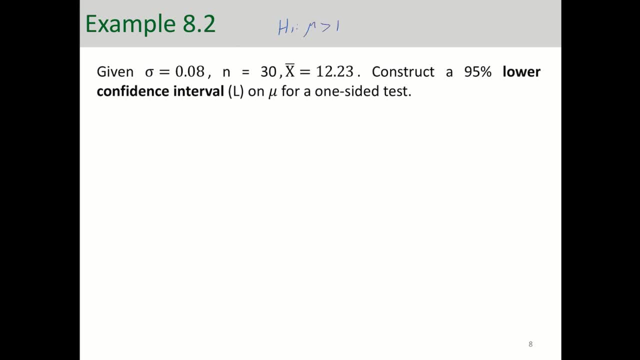 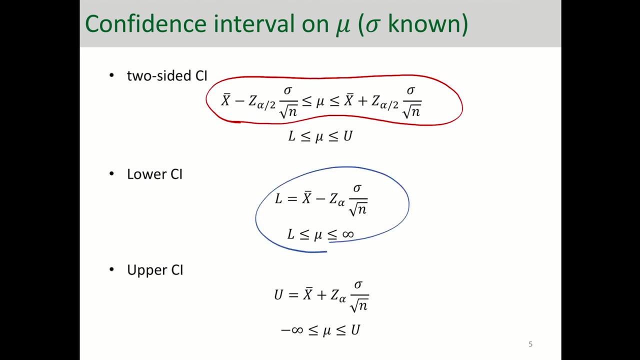 which was- It was probably mu more than- if you remember this example from before- mu more than 12.2.. Now we only want to find the lower confidence limit. If I go back a few slides back here, the lower confidence limit is here. 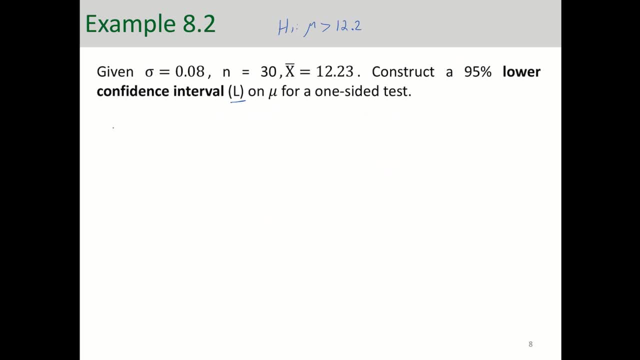 So we're going to use that formula. l is equal to x-bar minus z of, alpha sigma, square root of n, And here is 12.23 minus z of, because it's a 95% alpha is 0.05.. 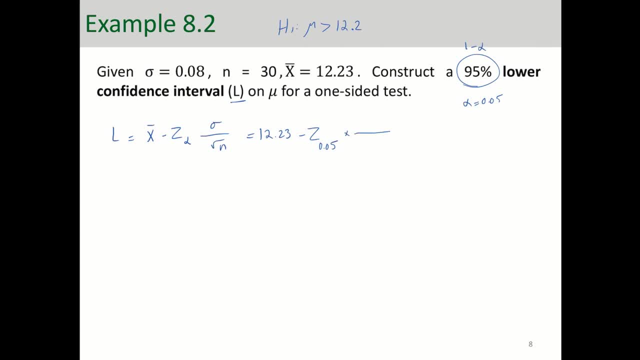 And here we have z of alpha times: 0.08 over square root of 30. And this value, if you read it from the table, that is 1.64.. And if I replace everything with numbers and do the math, I will get 12.2..